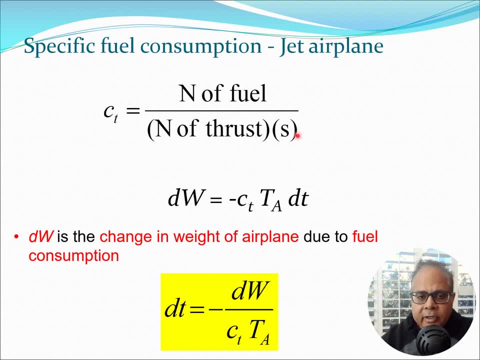 this particular fuel consumption for a propeller powered aircraft. So we are going to talk about particular nomenclature to get the value for dW. So dW is essentially the amount of fuel which is being consumed or dissipated And this is equal to Ct, into Ta, into dt. So what I have done here 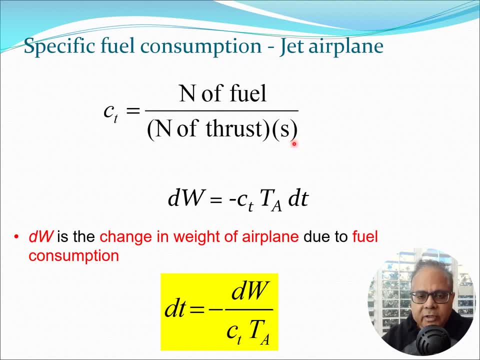 is. I have taken S as a measure of time, that is seconds, into dt. The newton of thrust has been taken into the available thrust And Ct is here, and the negative sign simply means that this is decreasing because of course, fuel is being expended by the jet engine. So dW or the weight, 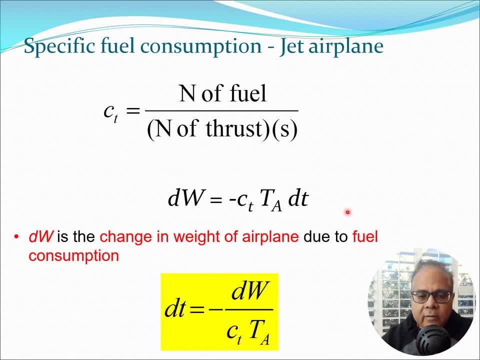 of the airplane is decreasing as you are going through time. So that is the physics behind this equation. So dW is the change in the weight of the airplane due to fuel consumption. So we can write this equation in terms of dt equals negative dW by Ct, Ta, And this equation is going to help. 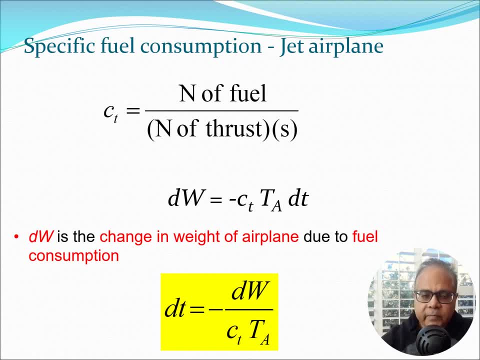 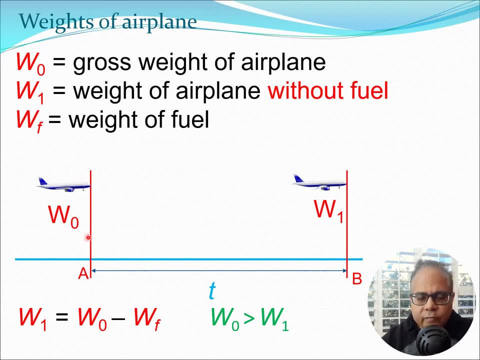 us get the value of time. So before we get there, let us look at the typical airplane. You already know. the airplane starts out with the weight of W0, which is called the gross weight of the airplane, And at the end of the mission it has a weight of W1, which is the weight of the airplane without fuel. So during 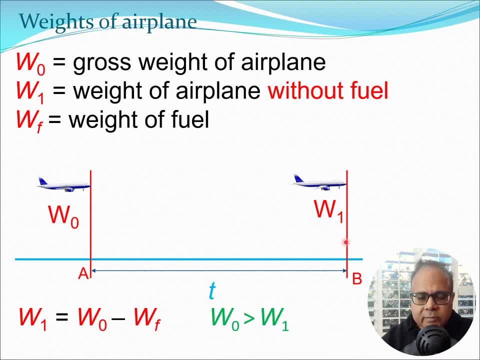 this journey from point A to point B. this fuel is expended, The weight of the fuel is Wf And what happens is that the time elapsed during this period is t. So this is the range. We can convert it to the range when we integrate all these small 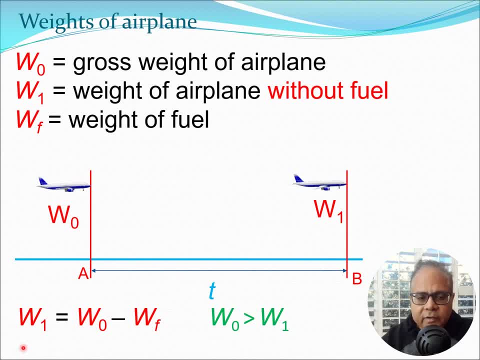 segments dt here. So some equations come out of this weight nomenclature. We know that W1 would be equal to W0 minus Wf, or at the end of the journey the weight is equal to the weight at the beginning of the journey minus the fuel weight. And this equation also immediately tells us that W0 is. 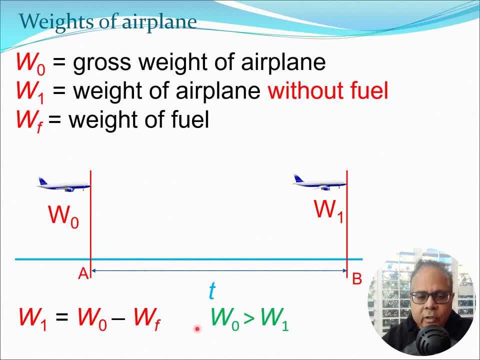 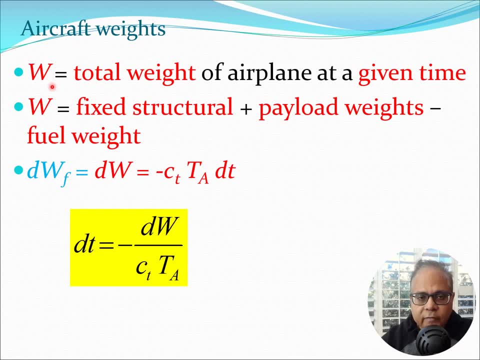 greater than W1, because W0 includes fuel, W1 does not include fuel. Now, one more nomenclature we had was W, which is the total weight of the airplane at a given time, And W is the fixed structural and payload weight. 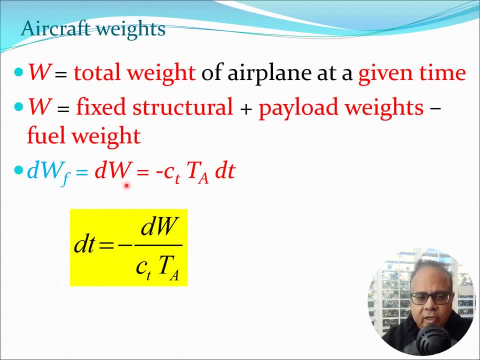 minus the fuel weight. So essentially dwf is equal to dw, And that was minus ct, ta, dt. So essentially when we say dw is same as dwf, we are making the point that the payload is fixed, the weight is fixed and so on. So hopefully no payload is being thrown, or 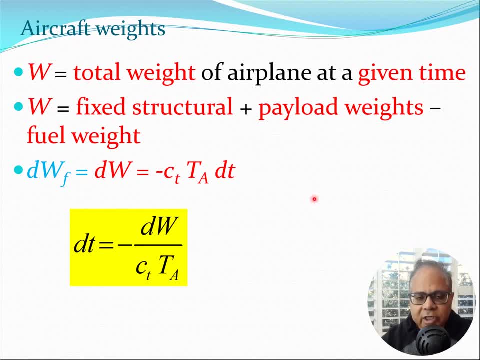 jettisoned during the flight. In that case, you would need to consider that in these equations. So let us get back to this equation. Now. we have a good understanding of the weights at the beginning and end of the journey, So therefore, I can take this equation for endurance, and I can 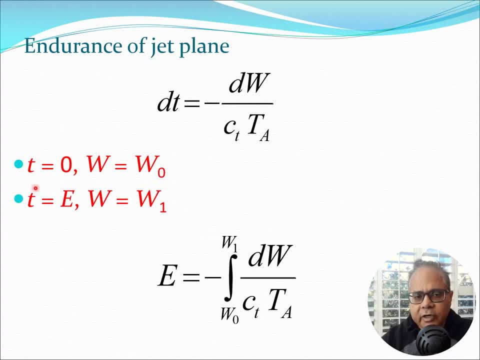 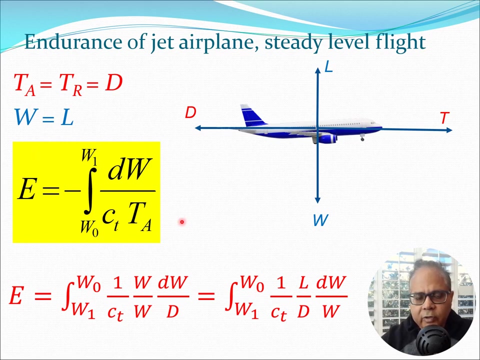 integrate it. So essentially, dt has to be integrated from t equal to zero Where w is w0, and t equals to e where w is w1, and this is the integral e. So this will give me this value here: w0 to w1, dw by ct, ta. Now, this particular value, we are going to expand it. 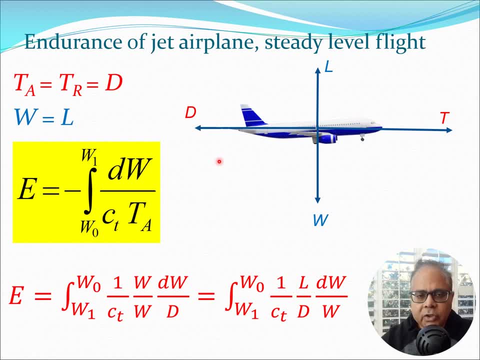 and simplify it because we want to now get closed form solution. So do recall that we are in steady level flight. So we are going to make that assumption that we are in steady level flight And therefore, during this flight, lift is equal to weight and thrust is equal to drag. So these are. 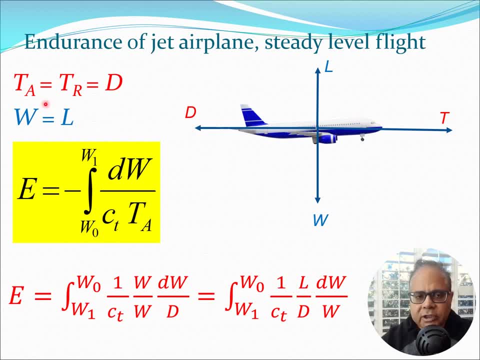 the basic equations. So we will also assume that ta is tr is d, So the pilot has enforced this condition. and also, weight equals to lift. So now from this equation, I can rewrite this equation in this form. So all I have done is I have substituted ta is d here, So I got this d here. 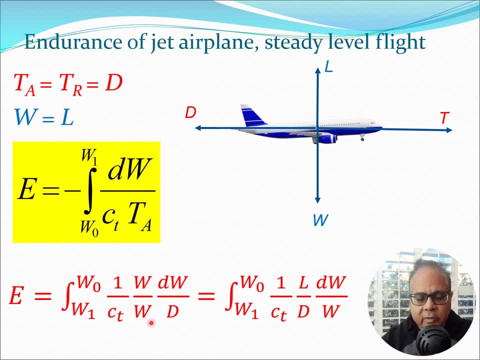 and I have multiplied the numerator and the denominator, So I have got this d here and I have multiplied the denominator both by w, So I got this w by w term, and also I have flipped this integral bound, So essentially I have absorbed the negative sign inside. So what has happened? 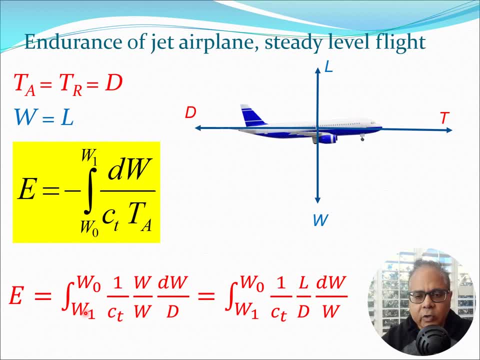 w0 has gone up and w1 has gone down. So this is something we can do from calculus. So now, with this particular integral, we make one more change. We know that weight is equal to lift, So I bring the drag, I put it here and I put this w in the place of drag. So by this rearrangement I get 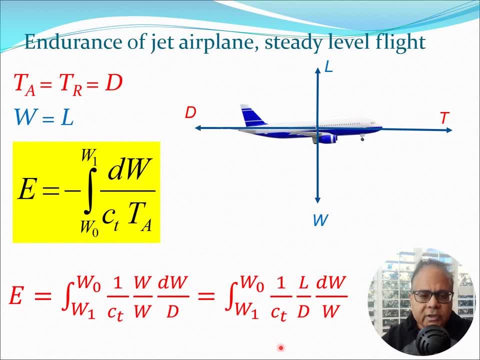 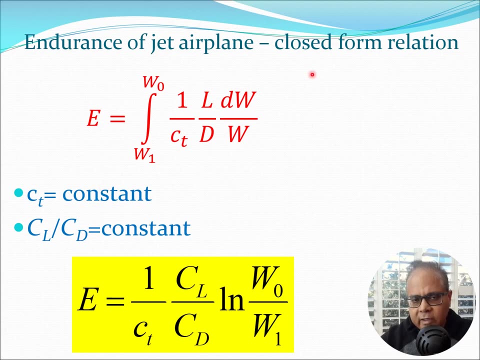 this nice looking equation here and now I have expressed things in terms of the weight, w, l by d ratio and 1 by ct. So this is the integral we are going to try to do. This integral is much more amenable for closed form solution. So now we take a look at this integral here and we assume that ct 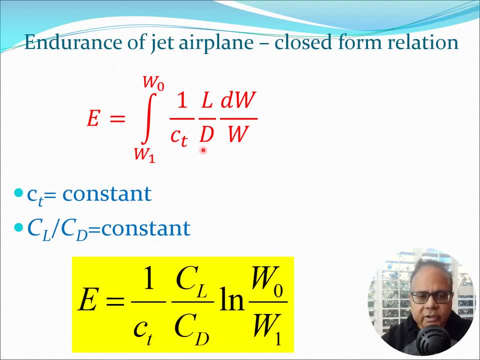 and if we do that, we can drag these two terms out from the integral to outside it, and then we are left with dw by w. Now you know, from calculus, the derivative, or rather the integral of that is log of w, and so I get log of w0 by w1 when I put these two bounds here. So this is the. 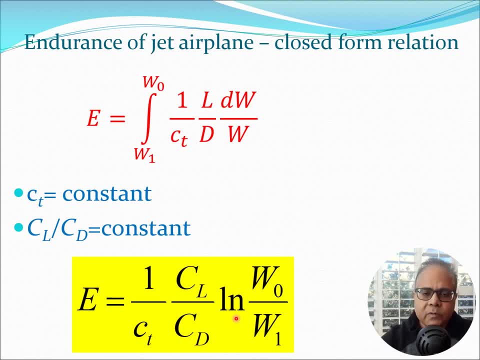 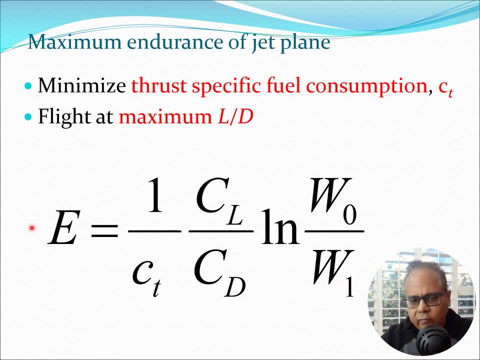 natural log to the base e. So this is the closed form solution for endurance of a jet airplane. So we try to always look at the math model and see what we can extract out of the model. This is one of the fundamentals in any kind of engineering research or study. So we look at this and let's 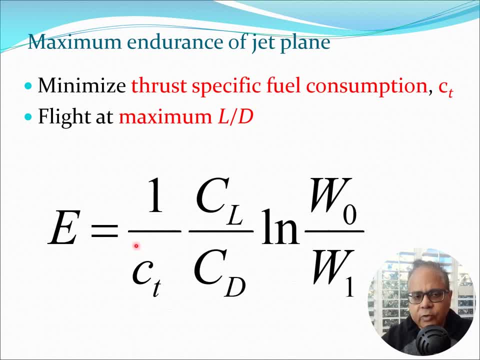 say how we could maximize e. We can of course see we could minimize ct, which would mean that I minimize the thrust specific fuel consumption. So that is a driver of the engine technology and so on. I would also want to fly at maximum l by d or maximum cl by cd. So again, that is something. 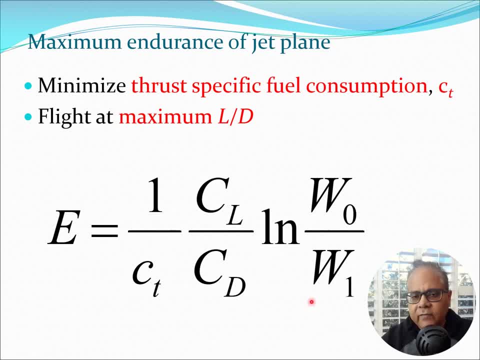 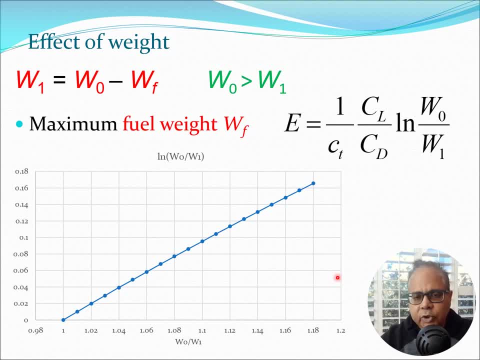 then the weight component I am going to look at in the next slide. So if we look at the weight part here, we will see that this w0 by w1 is always going to be more than one because w0 is greater than w1.. So if I were to plot this here, I have plotted. 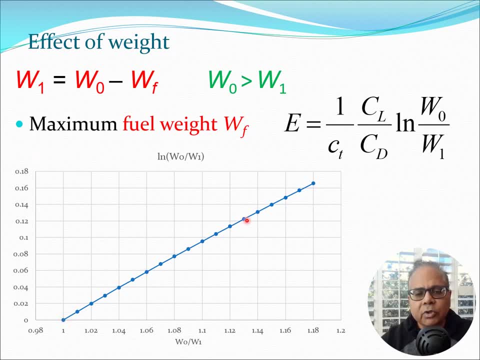 W 0 by W 1 versus log of W 0 by W 1, starting from 1.. So this always goes up like this. So if we look at this now, So if we were to look at the weight data of the early stage, we will see that this much E0 by E1 becomes 10 over 1.. So if we have thisicherung will be. 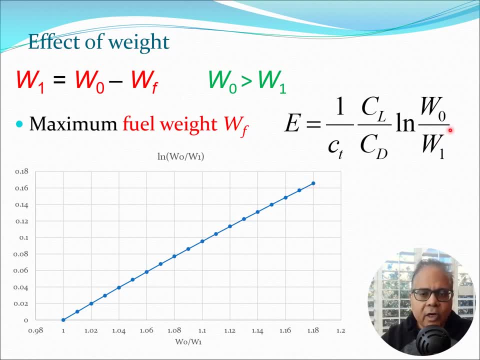 up like this. So, essentially, I want this value to go up, and for this value to go up, what I need to do I need to have a higher value of fuel weight. So the higher value of fuel weight will ensure that this particular endurance keeps going up. Now, of course, there are limits to that in terms 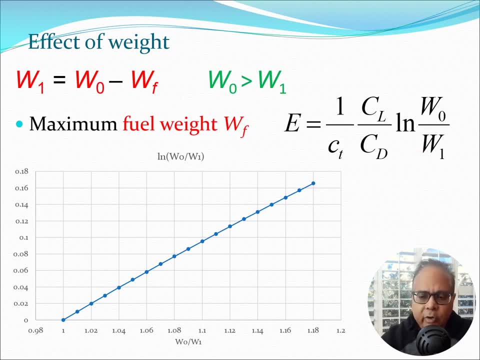 of the structures in terms of cost, in terms of the aerodynamic performance and so on. but it is something which comes out of common sense that you need to have a bigger fuel tank if you want to have more endurance. That's something you would even know if you are somebody who drives a. 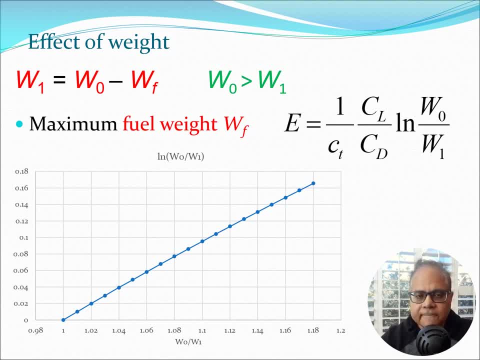 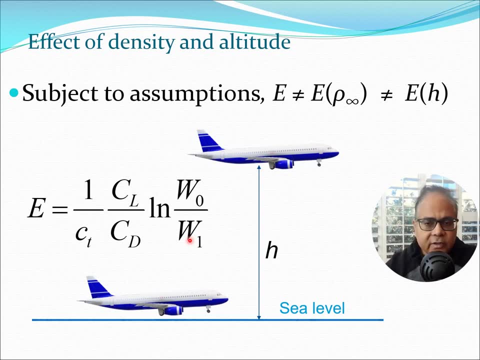 car or an SUV or a truck or something like that. So now let's again take a look at the equation. From this equation we can see that, subject to the various assumptions we have made, the endurance is not a function of density and therefore it should not be a function. 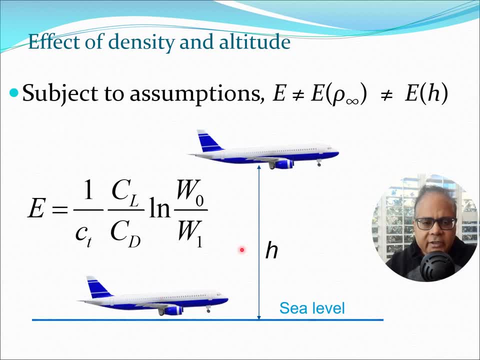 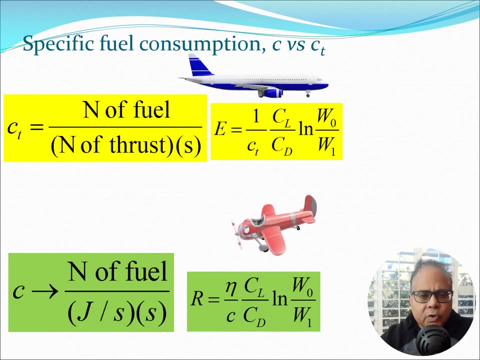 of altitude. Therefore, if I am flying the aircraft at sea level or I am flying it at some height here, edge, The endurance of the aircraft should not be impacted, because those things are not directly coming into the equation here. So just to recapitulate: today we looked at the specific 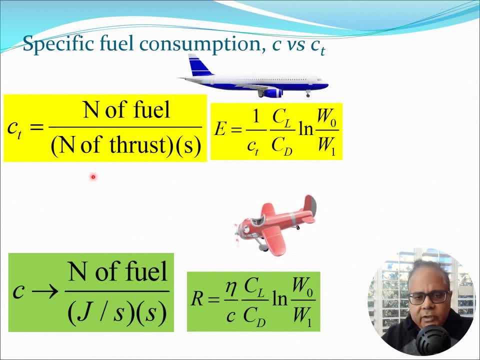 fuel consumption, ct, and this was defined in terms of thrust. So this is what is used for the jet engines. Previously we used the c for the propeller engines, and that was defined in terms of power, which was joule per second here. So in that case we were able to get the expression for range for a propeller aircraft as this, and now 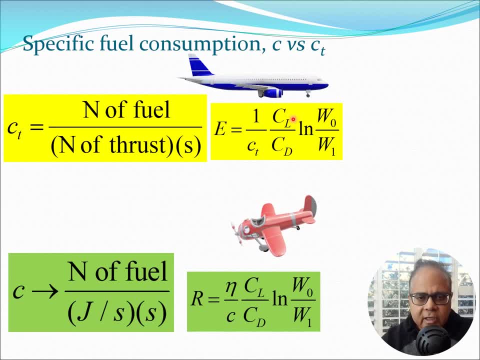 we get the expression for endurance for a jet aircraft like this. Now, these two equations look somewhat similar, but there are some differences here. The efficiency of the propeller is coming in here. Now, if you look at the units, you will see that cl, cd, all these are dimensionless, w0 by w1.. 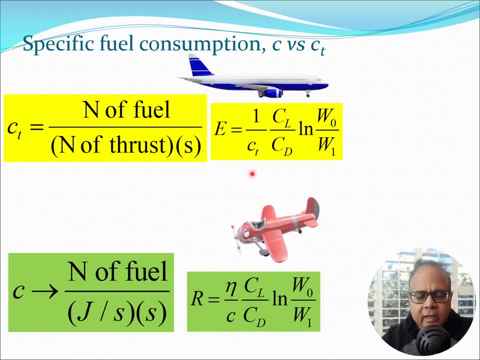 So the unit of this is governed completely by ct and the unit of ct is actually newton by newton and second here. so one by ct. So one by ct means the endurance is coming out in seconds. If we see here, you will see that this is joule per second into second, or this is essentially 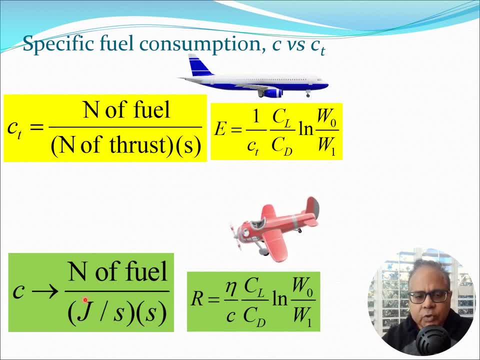 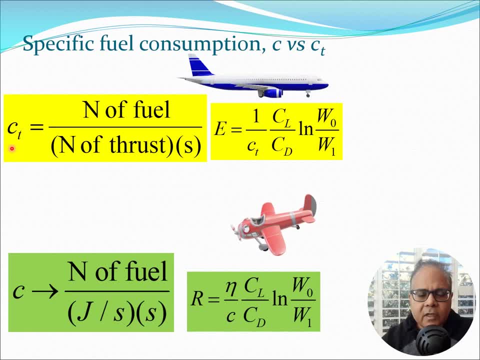 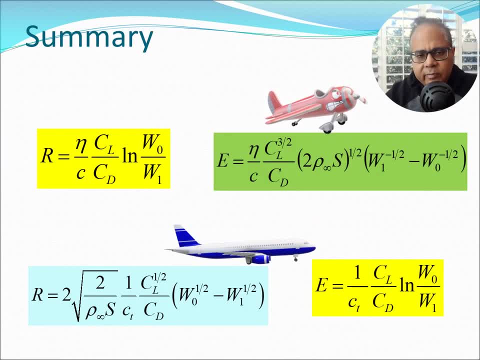 of different units. So finally, to summarize, we will see that the different endurance and range of different aircraft are given here. So for the propeller we obtained in the previous two classes, range is given by this thing in yellow, endurance in this box in green. 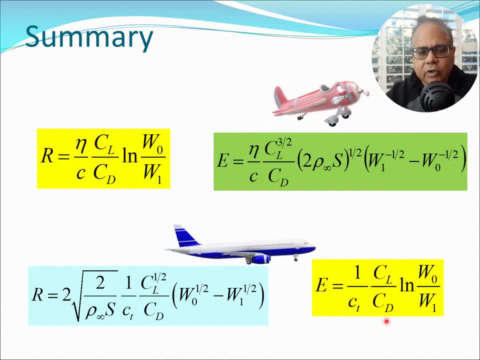 And for a jet the endurance is given by this box in yellow here. So you can clearly see there is some analogy between the endurance equation and the range equation for the jet and the propeller respectively. So in both these cases cl by cd has to be maximized during. 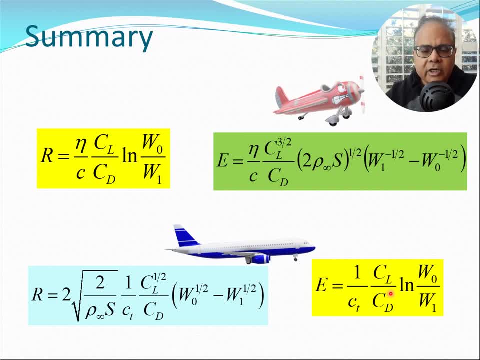 the flight. So that is the driver. as far as the aircraft performance is concerned, If you want to maximize endurance, you have to fly it such that cl by cd gets maximized for the jet And for the propeller. again, you want to maximize range, you want to fly it at the point where 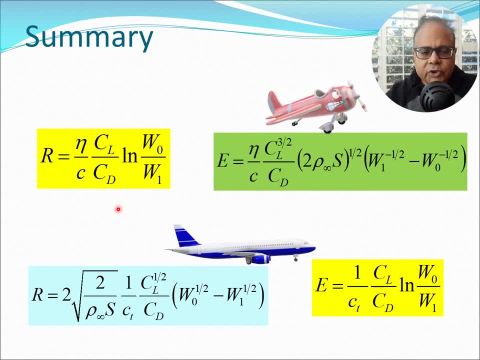 cl by cd gets maximized for the propeller. So now the thing which remains is range of the jet, and that is this equation. here That is something quite different. It is directly related to cl- half by cd- and we are going to derive this in our next lecture. 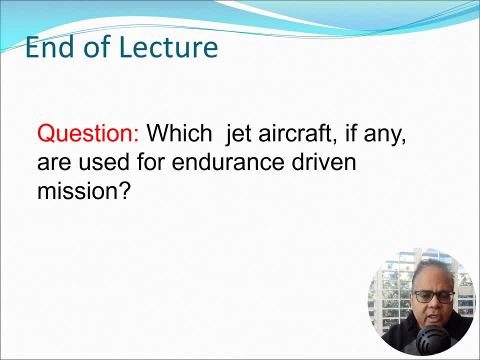 So this is an interesting question I have for you that, in case you know that you are going to know about different type of aircraft, try to figure out: are there jet aircraft which are designed for endurance driven missions? So that is something which is interesting to know. 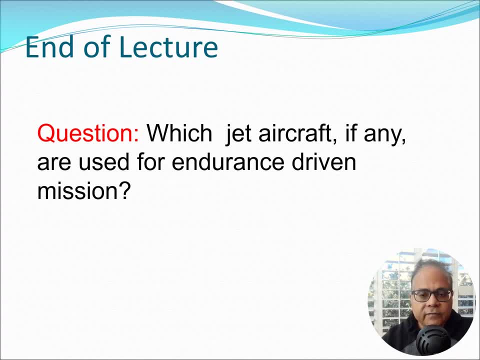 I will stop this video now. I will see you in my next video, when we are going to talk about the jet aircraft again, and then we are going to discuss range, which is a very important problem, because most often jet aircraft are used to fly between two cities, and sometimes 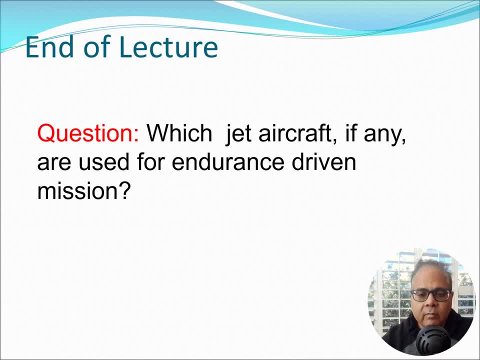 two cities can be very far away, So you can even travel today from Bangalore to San Francisco, for example, in a direct flight. I will end this video now and I will see you in my lecture soon. See you then.